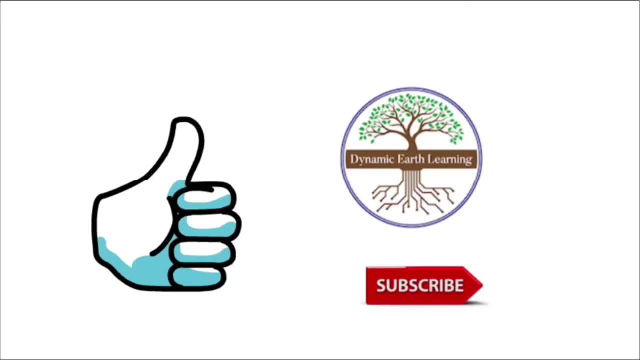 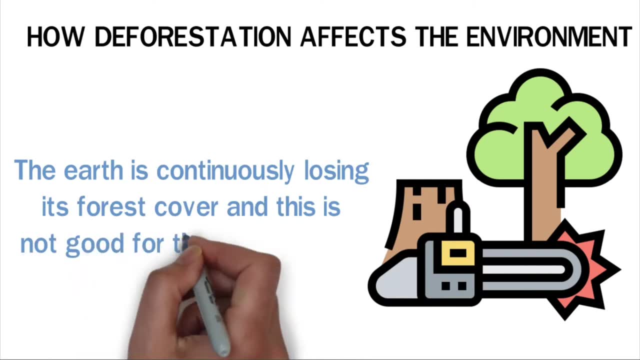 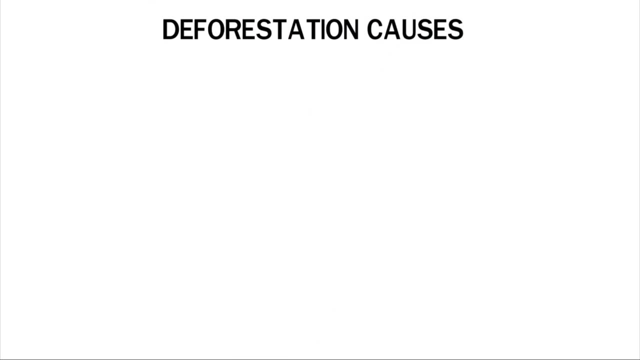 for more science and sustainability videos. You can also check out our blog and online courses in the links in the description. The Earth is continually losing its forest cover and this is not good for the environment. Deforestation causes. Deforestation can occur due to several reasons. When trees are deliberately cut to create room for other activities, it 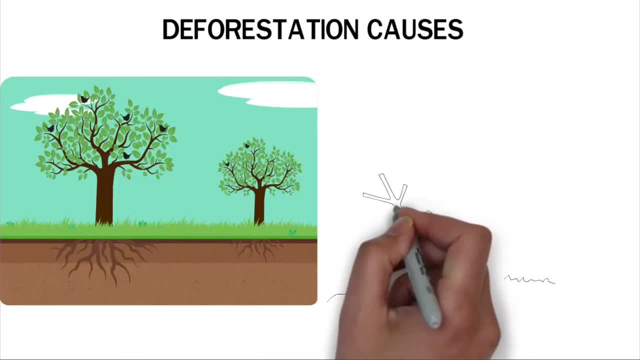 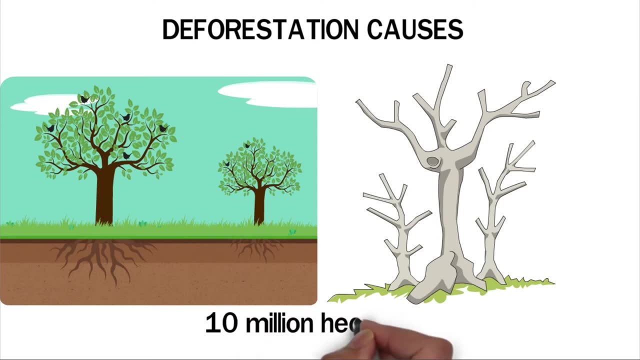 causes deforestation. Certain accidental disasters can also lead to the loss of forest cover. It is estimated that the Earth loses 10 million hectares of forest cover in just a few days. The Earth is also losing 10 million hectares of forest cover every year due to the following. 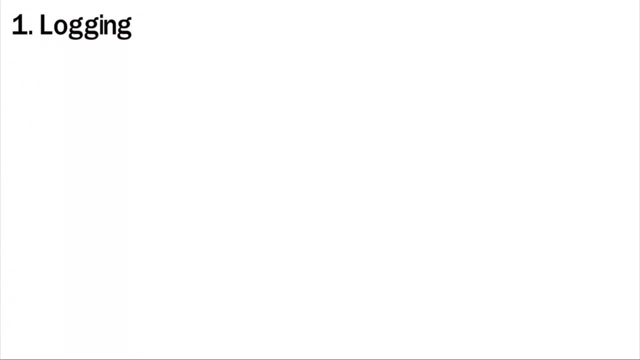 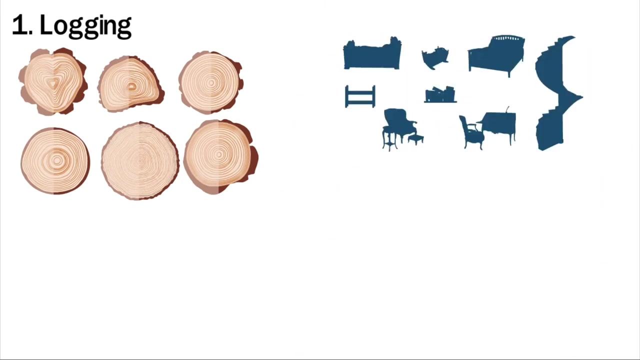 causes: 1. Logging Trees are a source of wood which is used as fuel locally. A large percentage of forest cover is lost every year from charcoal burning. The furniture industry also uses timber when making chairs, tables, building materials and other wood products. Since paper. 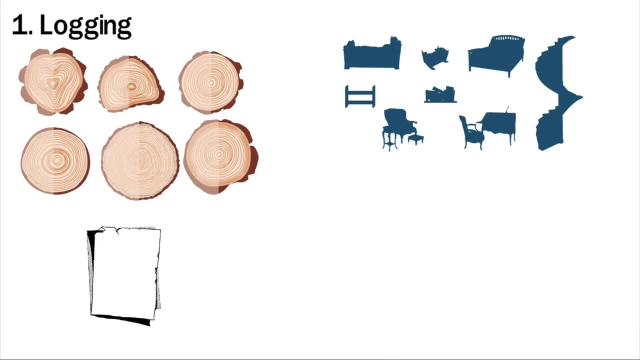 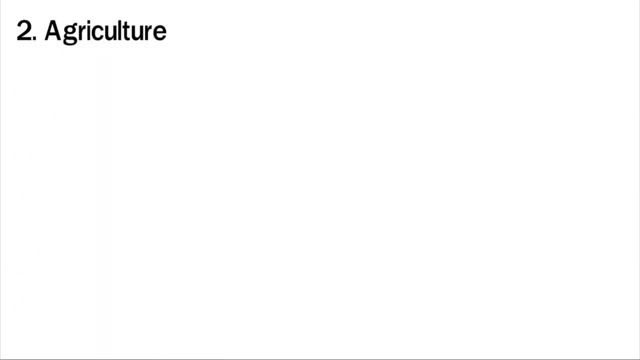 is made from wood, trees have to be cut to obtain the needed materials. Most of these industries practice illegal logging, thereby destroying forest cover. 2. Agriculture: Up to 80% of deforestation around the tropics is caused by agricultural activities. As the human population continues to grow, the demand for food increases. People 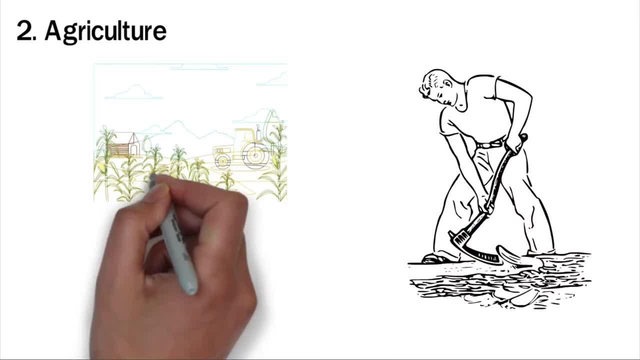 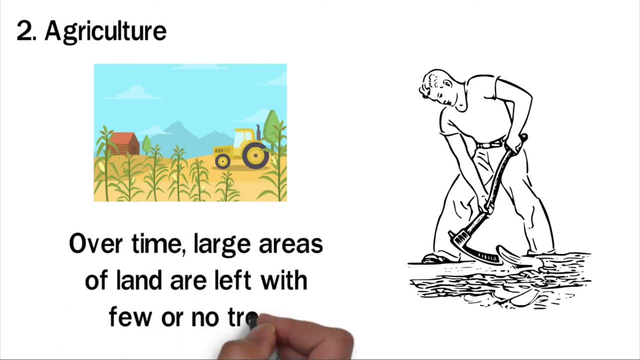 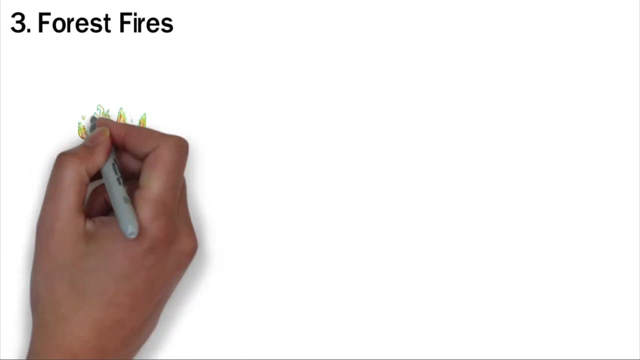 have to cut down trees to create space for crops. Trees that are cut for this purpose are rarely replaced, leading to the loss of more forest cover Over time. large areas of land are left with few or no trees. 3. Forest fires. Each year, the Earth loses trees due to forest fires. For example, the 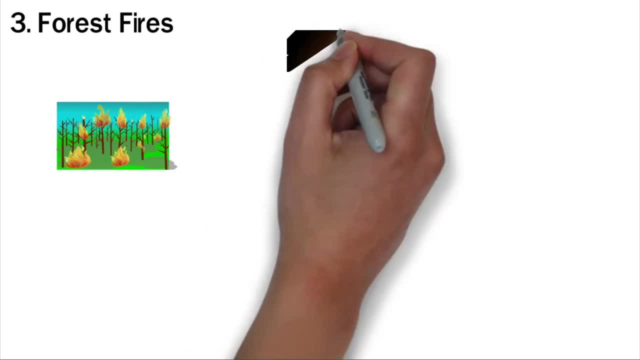 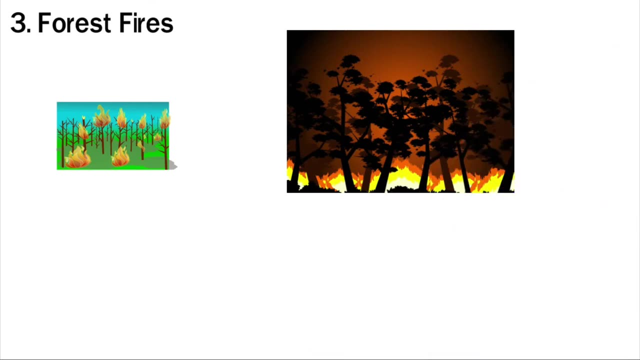 forest fires can result from human activities or natural disasters. People often start fires in a small area when clearing land for other activities. If the fire is not controlled, it can spread to forests. Also, forest fires can be caused by extreme weather conditions. 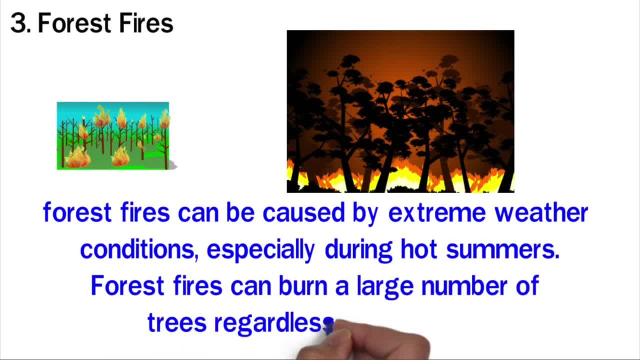 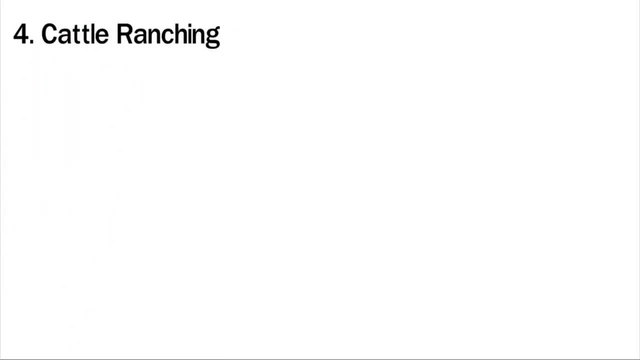 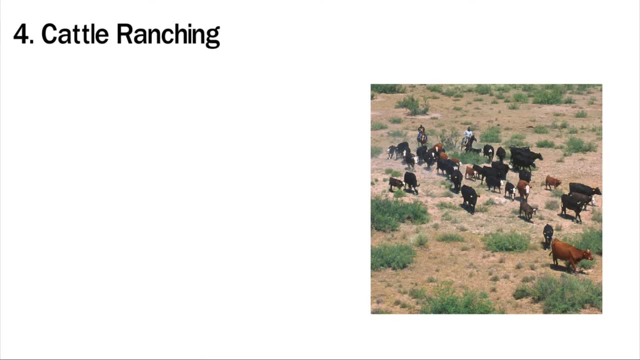 especially during hot summers, Forest fires can burn a large number of trees regardless of the cause. 4. Cattle ranching. Cattle ranching is the main cause of deforestation in the Earth's tropical rainforests. Large areas of forest cover have been cleared to create room for ranching activities in 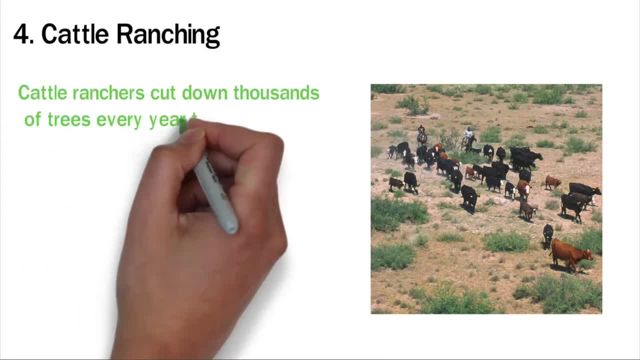 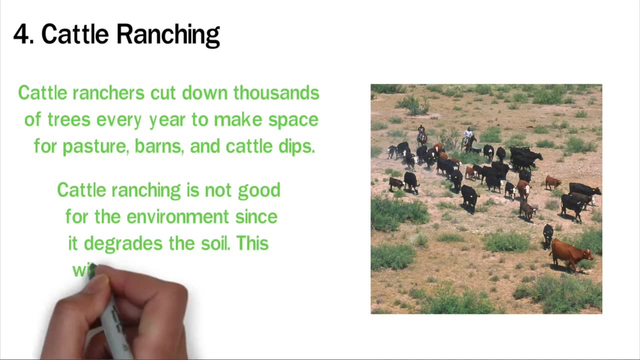 different parts of the world. Cattle ranchers cut down thousands of trees every year to make space for pasture barns and cattle dips. Cattle ranching is not good for the environment, since it degrades the soil. This will prevent trees from growing as they should. 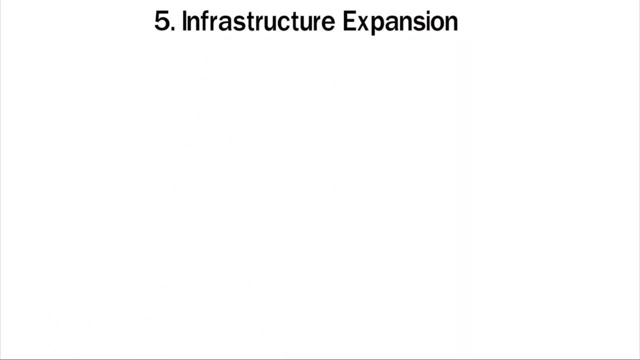 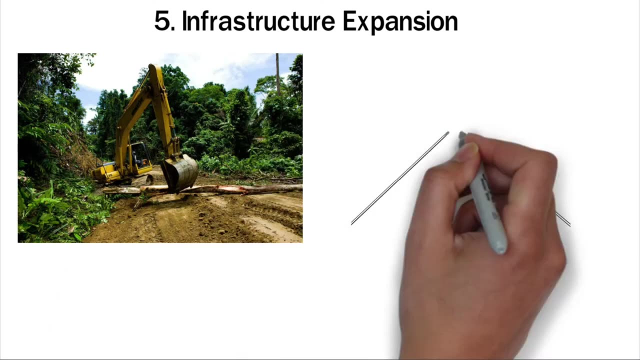 5. Infrastructure expansion. Due to urbanization, trees have to be cut to make room for buildings. Trees are also cut down when constructing roads. Roads that pass through or near forests can cause massive deforestation in a given area. Other features, such as dams, may also. 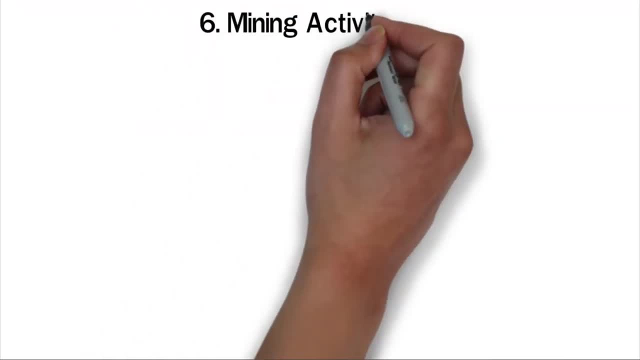 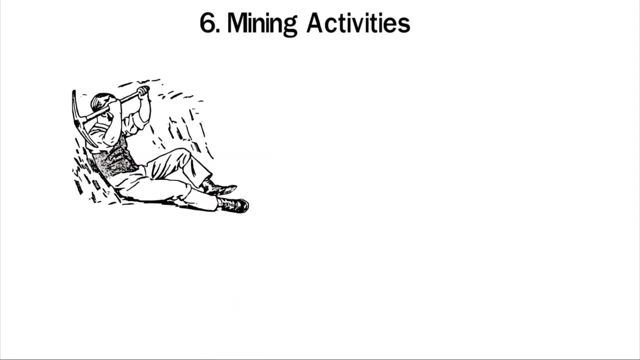 require the felling of trees. 6. Mining activities. Mining is the extraction of minerals, metals and other geological materials from the soil. These activities can greatly impact forest cover. To excavate these materials from the Earth, the forest cover has to be cleared. This leaves the soil. 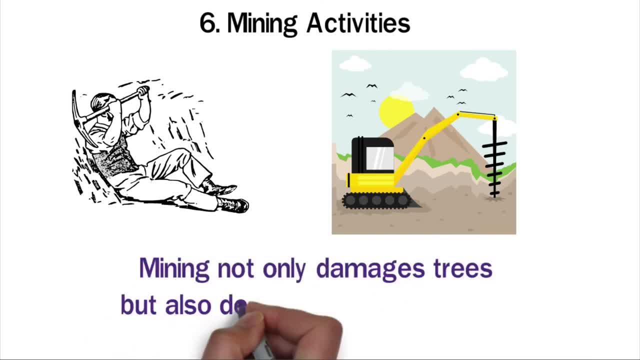 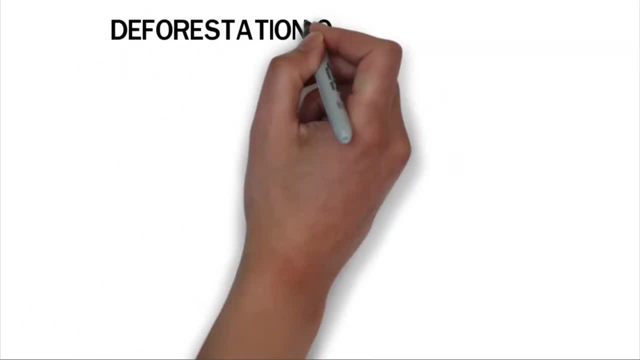 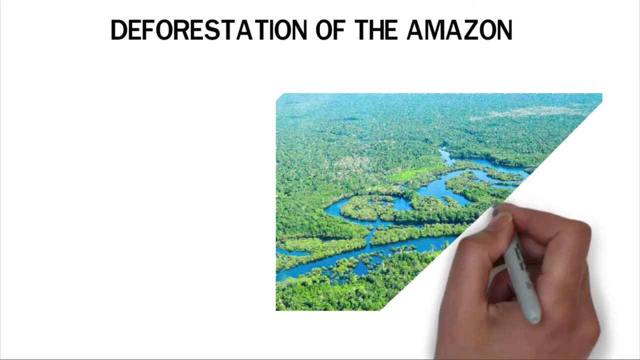 also damage trees. Mining can also damage trees. Mining can also damage trees. Mining can also damage the trees that you're burning. 6. Deforestation of the Amazon- Definitely the largest rainforest in the world. the Amazon is undoubtedly the largest rainforest in the world. It covers less than 4% of the. 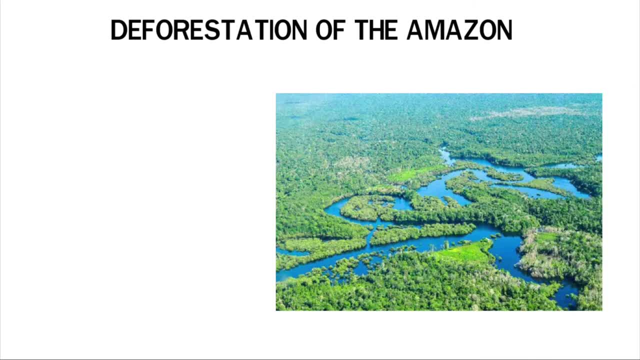 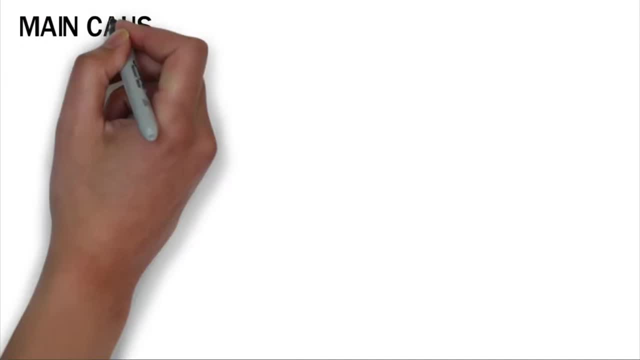 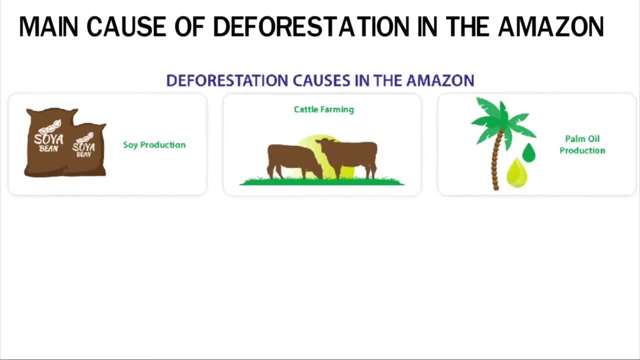 Earth's surface and creates approximately 20% of the Earth's oxygen. The Amazon rainforest is continuously shrinking due to deforestation. 7. Main cause of deforestation in the Amazon. Like most rainforests found in the tropics, the main cause of deforestation in the Amazon. 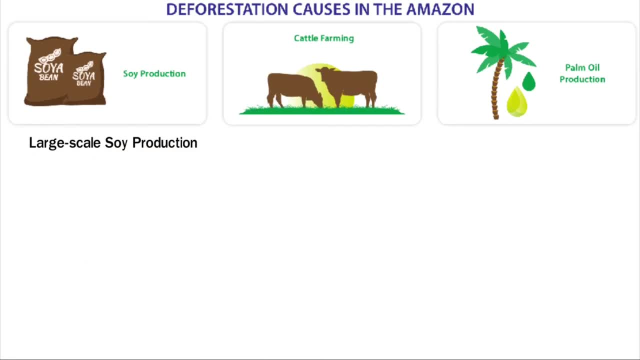 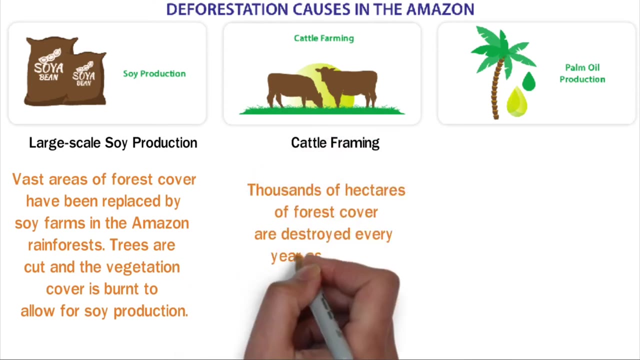 includes Large-scale soy production. Vast areas of forest cover have been replaced by soy farms in the Amazon rainforests. Trees are cut and the vegetation cover is burnt to allow for soy production Cattle farming. Thousands of hectares of forest cover are destroyed every year as a result of cattle ranching in the Amazon. 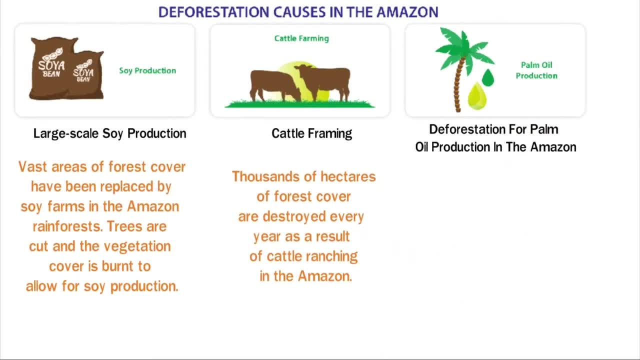 Deforestation for palm oil production in the Amazon. Besides soy, the trees in the Amazon were cut to make way for palm tree plantations. Palm trees produce palm oil, a type of vegetable oil that is used as biofuel. Palm oil can also be used in the cosmetic and pharmaceutical industries. 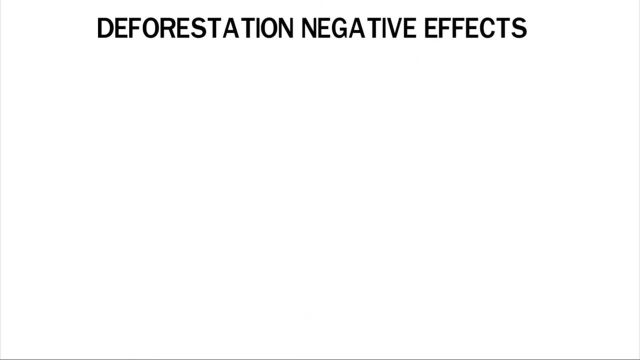 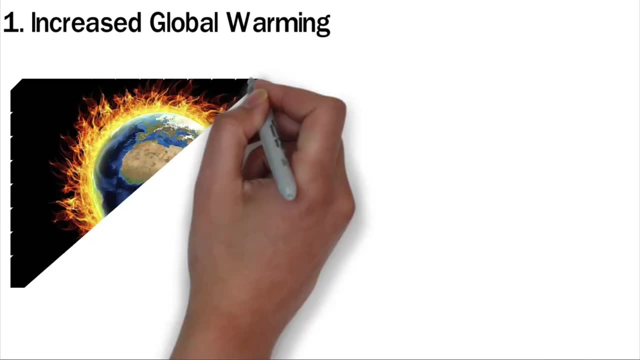 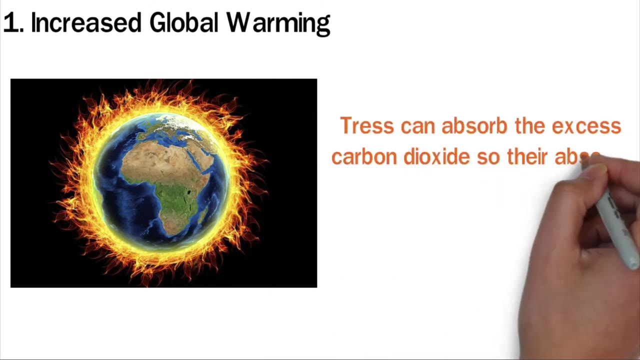 Deforestation negative effects. Deforestation impacts the environment in several ways. 1. Increased global warming. Global warming is the gradual increase in temperature in the Earth's atmosphere. This effect is attributed to increased carbon dioxide levels. Trees can absorb the excess carbon dioxide. 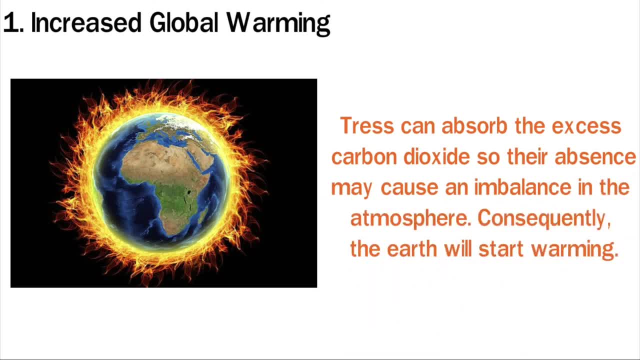 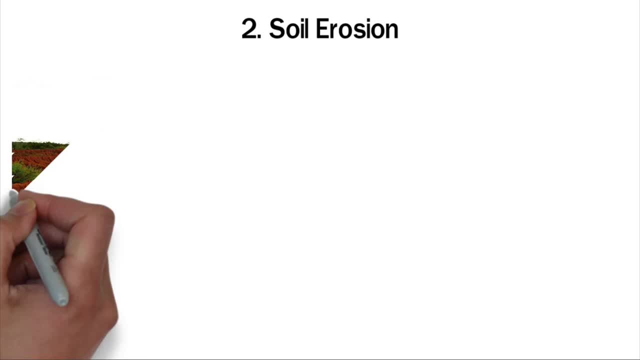 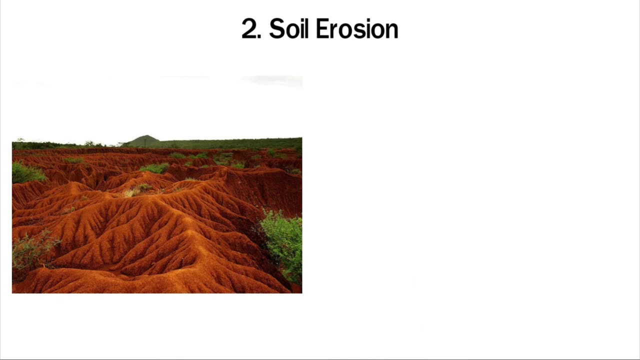 so their absence may cause an imbalance. consequently, the Earth will start warming. 2. Soil erosion. Trees provide coverage to the soil, thereby preventing soil erosion. When trees are cut, the soil is left exposed to the agents of corrosion. Soil particles are held in place by tree roots. 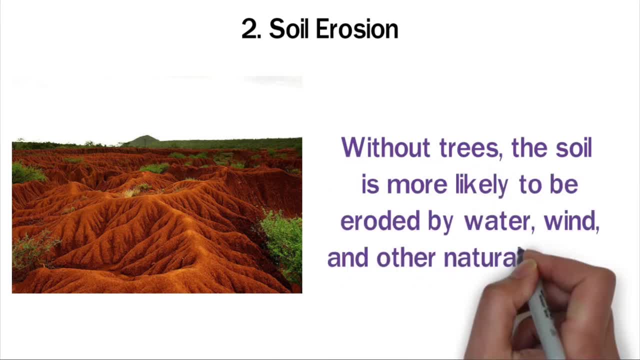 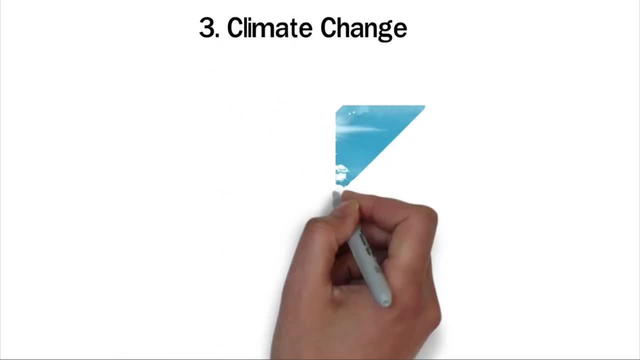 Without trees, the soil is more likely to be eroded by water, wind and other natural agents. 3. Climate change: Deforestation has many negative effects on the climate. Trees are an essential component of the water cycle. They absorb water from the soil and release it into the atmosphere. 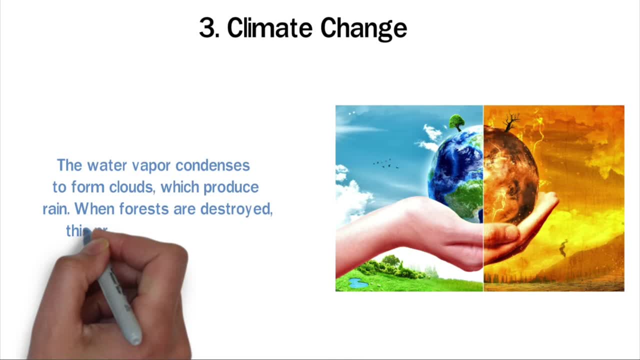 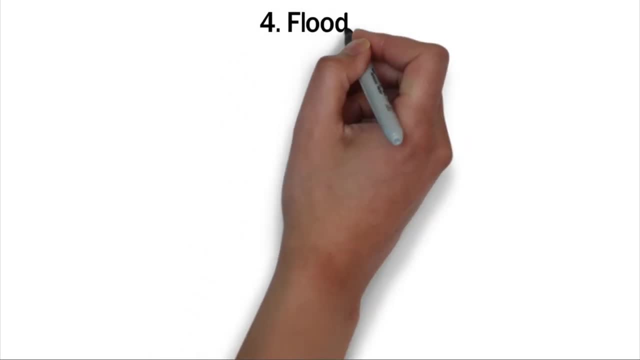 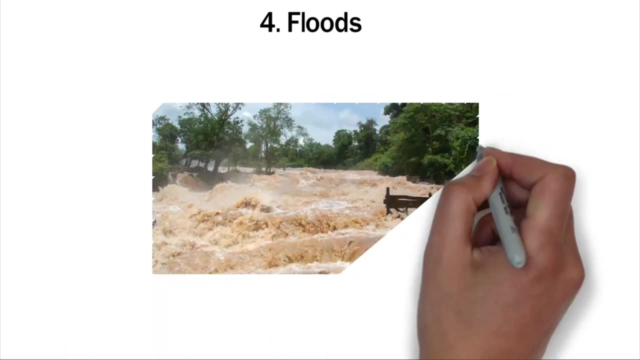 The water vapor condenses to form clouds which produce rain. When forests are destroyed, this process is interrupted, causing a change in climactic conditions. 4. Floods Without forest cover: the soil will have poor drainage. This can cause surface runoffs, leading to floods in the affected areas. 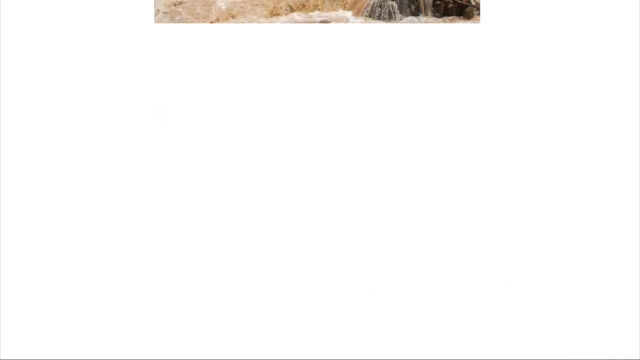 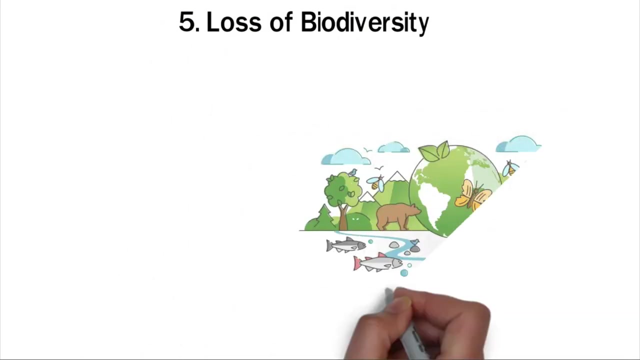 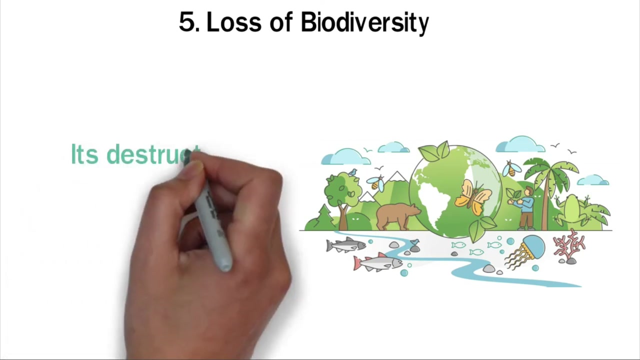 Floods can destroy property and may even cause death in worst-case scenarios. 5. Lost Loss of biodiversity. Rainforests provide shelter to different species of animals. Deforestation can lead to the loss of habitat and extinction of certain animals. The Amazon houses up to 10% of all animal species on Earth. 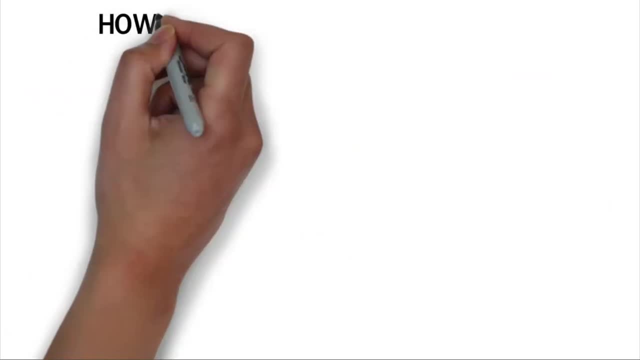 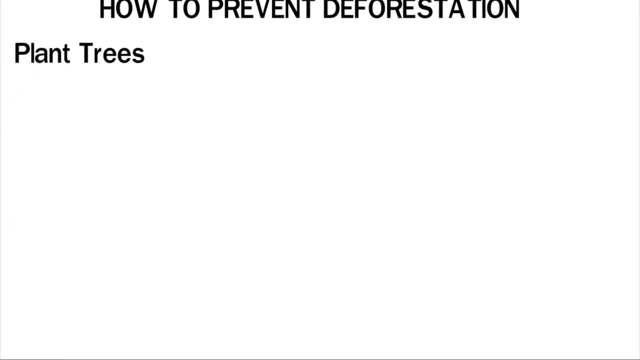 Its destruction could lead to serious environmental problems. How to prevent deforestation. There are different strategies that we can use to prevent deforestation. Plant trees. Trees are essential for the environment. By planting trees, we can avoid some of the problems listed above. 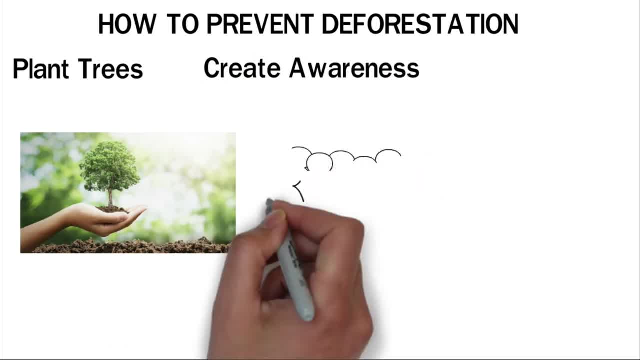 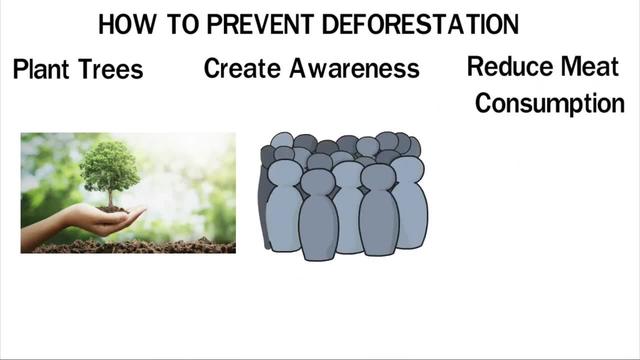 6. Create awareness. Most people don't know the effect that deforestation has on the environment. With proper education, people will learn how they can preserve forests. 7. Reduce meat consumption. Meat production requires a lot of space. This means forests have to be cut down to get the required space. 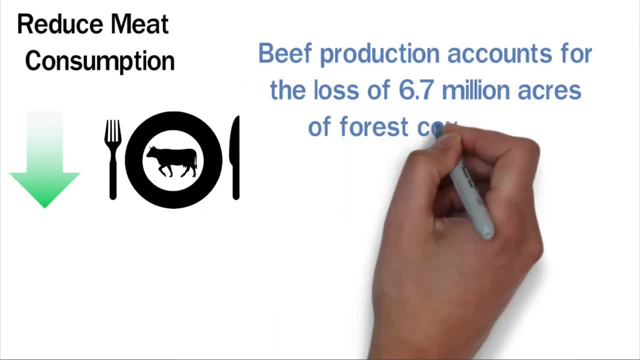 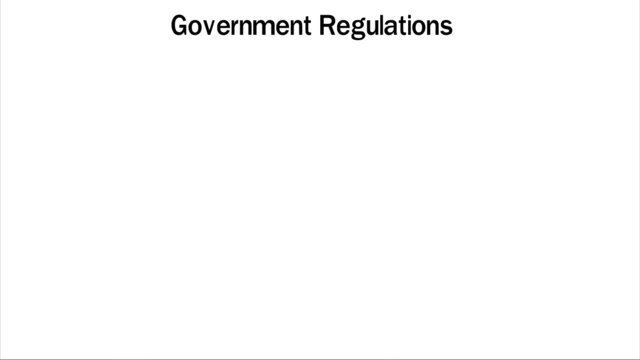 Beef production accounts for the loss of 6.7 million acres of forest cover in the tropical regions each year. 8. Government regulations: The government should impose regulations against illegal logging in forests. 9. Create awareness. This will greatly reduce the number of trees that are cut. 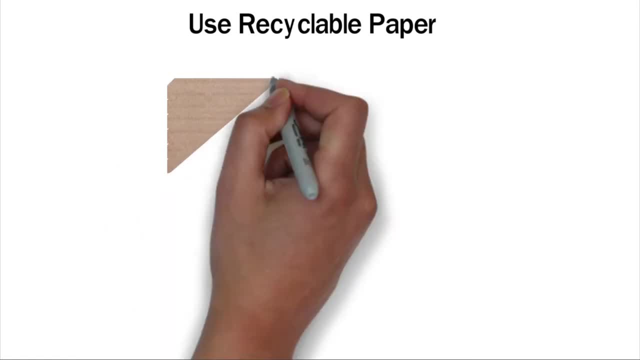 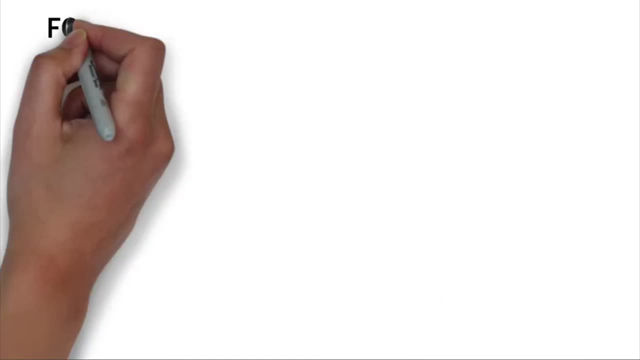 10. Use recyclable paper. When we use recyclable paper, trees won't be cut from time to time to make new paper. People should also use recyclable packaging materials. Forests are the lungs of planet Earth. Without forests, life on Earth would not be as we know it.